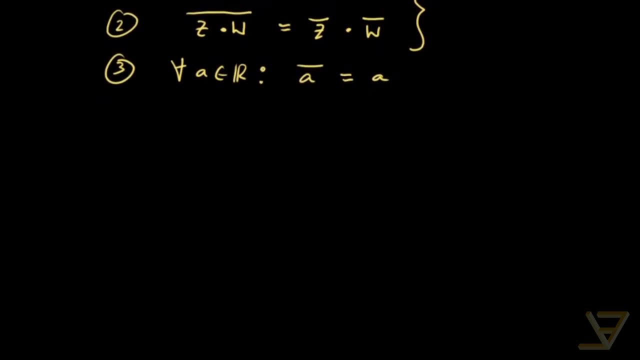 Because if we're flipping it over the x-axis but it's on the x-axis, then it just stays on the x-axis. Now here's the theorem that we want to be looking at. Let f be a real polynomial. Then, if z is a complex number, 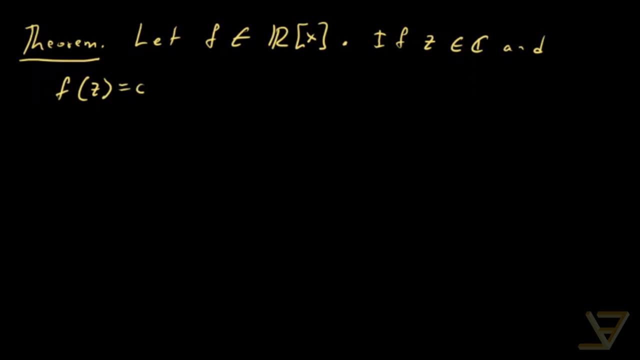 such that f of z is equal to zero. So z is a root of f. Then f of z bar is also equal to zero. So the complex conjugate is also the complex conjugate of the root. z is also a root. That means that if we were to 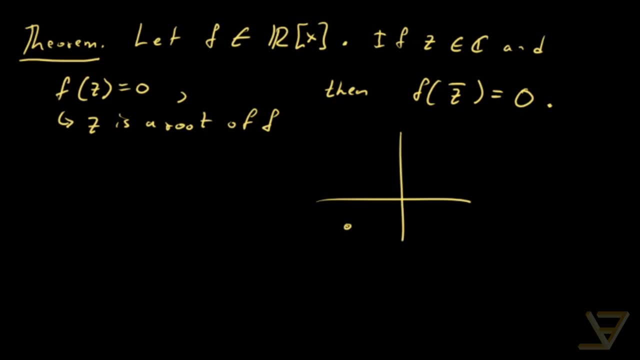 plot all the roots on the complex plane then by flipping them across the x-axis roots as well. So there are roots over here, here, here and here, because we've flipped them across the x-axis. But it should be noted that this is only true. 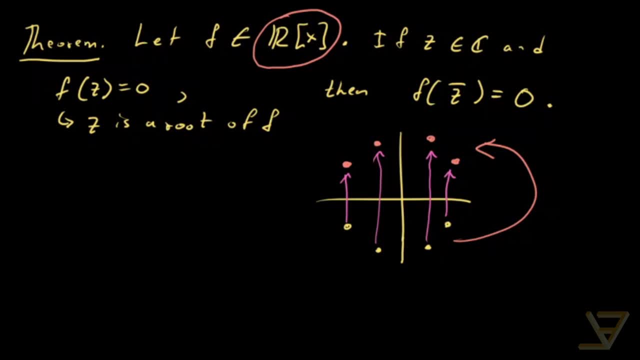 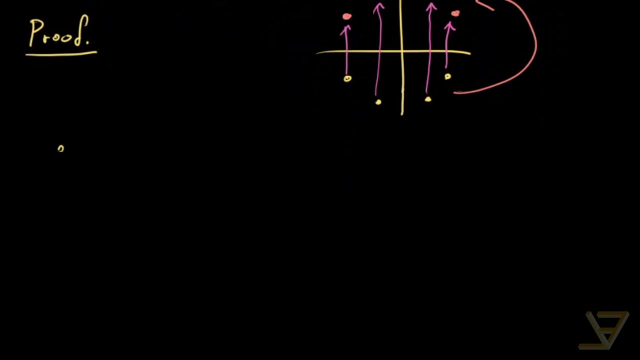 if we have real coefficients. If we have arbitrary, complex coefficients, this might not work. So let's prove it. Let's say that f of x is equal to a n. x to the n plus a, n minus one, x to the n minus one. 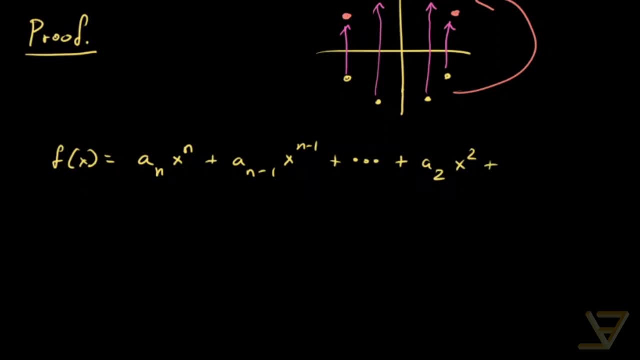 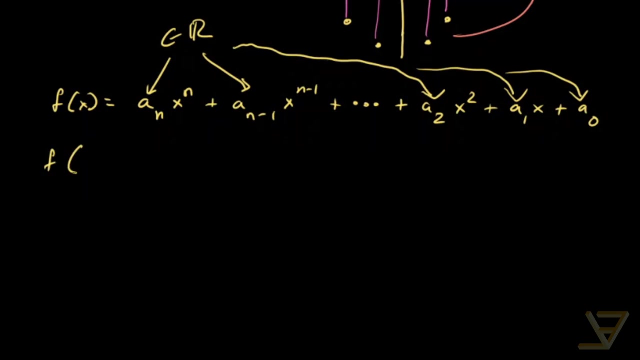 all the way through to a two x squared plus a one x plus a nought. Now we're going to have a chain of substitutions. But note that here we have the coefficients. All of these coefficients are in the real numbers. So let's say we substitute in. 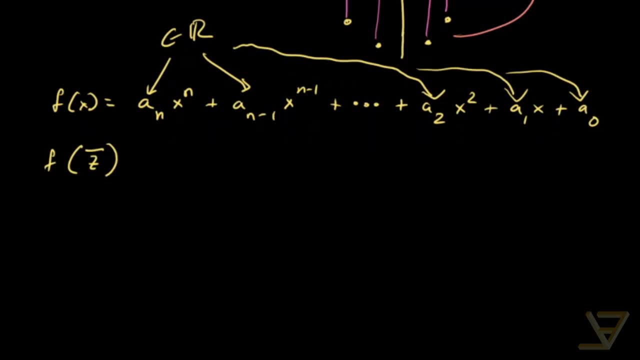 f of z bar. assuming that f of z is equal to zero, What we get is that a n z bar to the power of n plus a n minus one z bar to the power of n minus one, all the way through to. 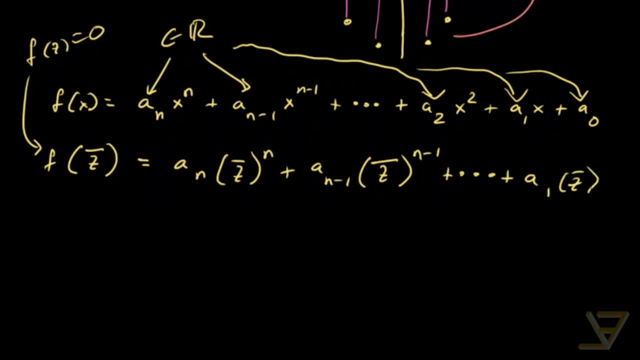 a one z bar plus a nought, And now we can take the bar to the outside of this parenthesis. So we get a n z bar to the power of n? Sorry, we get z to the n bar. 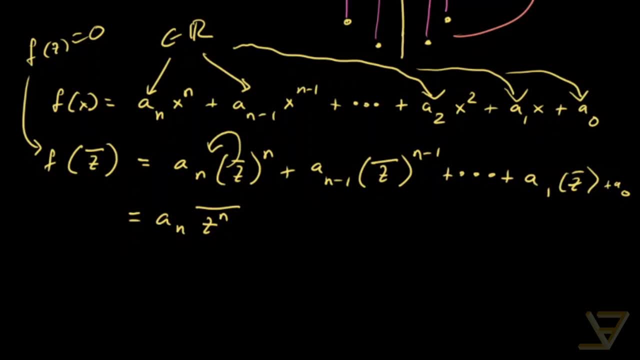 So we're taking, we're exchanging the conjugate with the exponent Plus a n minus one z to the n minus one bar, All the way through to a one z bar plus a nought. And now we're going to use the fact that 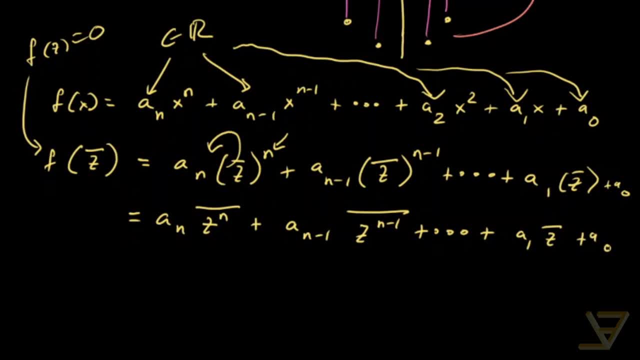 we can extend the bar over the real, the real coefficient, Because the conjugate distributes over minus one z to the n minus one bar. So we get a n minus one z to the n minus one. 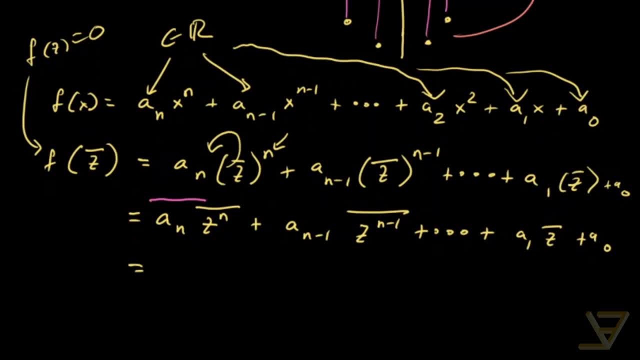 bar All the way through to a one z bar plus a nought. Now we're going to take a bar over the whole thing, because the conjugate distributes over the real number plus a nought bar. 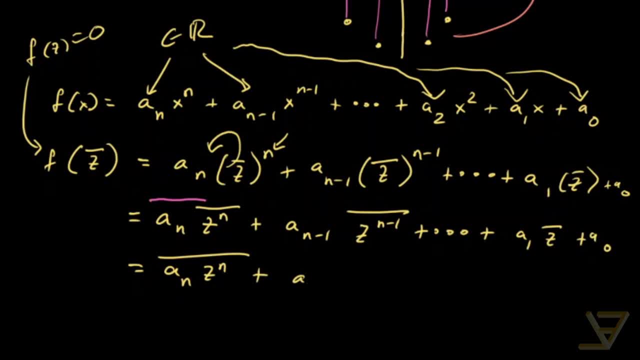 So we get a n? z to the n bar Plus a n minus one z to the n minus one bar, All the way through to a one z bar Plus a nought bar. 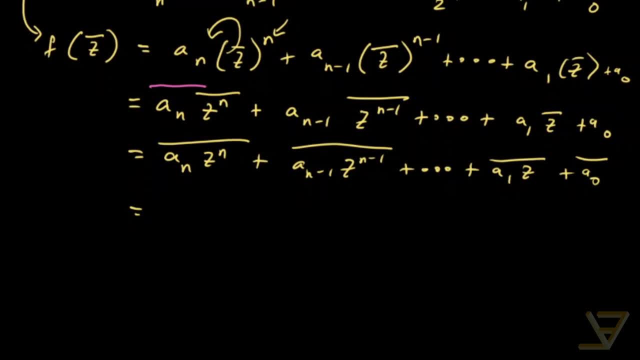 Now we're going to take a bar over the whole thing, because the conjugate distributes over addition. So we get a n z to the n plus a n minus one z to the n minus one plus. 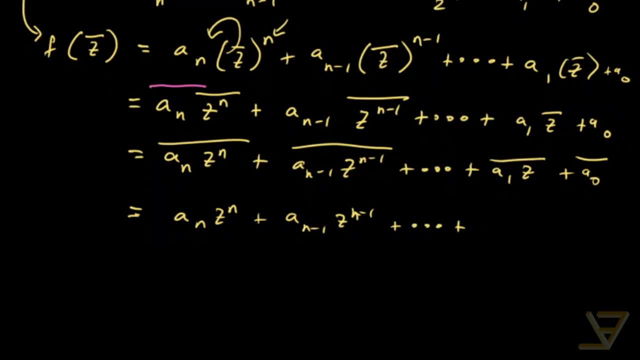 all the way through to a one z plus a nought And there's a bar over the whole thing. But this is just f of z bar, And that's equal to zero bar, And that is just equal to. 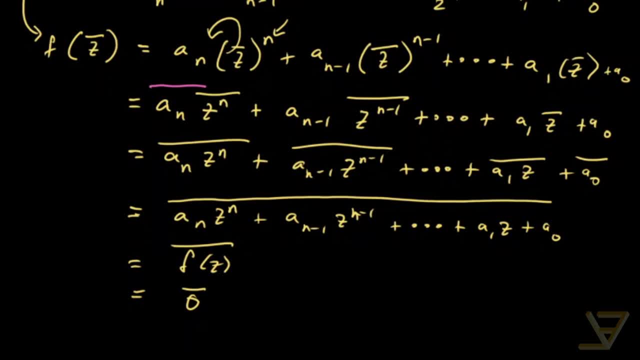 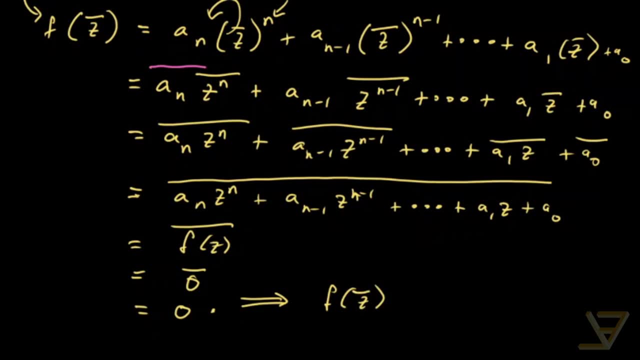 zero. So that proves a n minus one z bar plus a n minus one z to the n minus one. that proves that f of z bar is equal to zero. So z bar is a root. 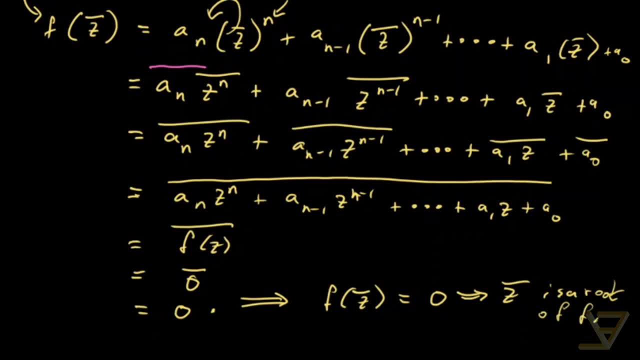 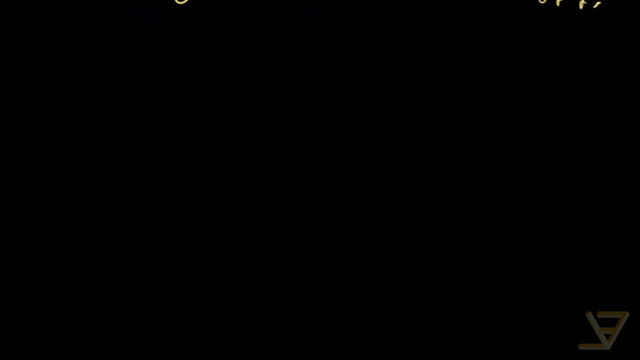 of f. So that proves that theorem. I just want to show you an analog in terms of rational numbers. So say, g is an element of the polynomials in the variable x with rational coefficients. 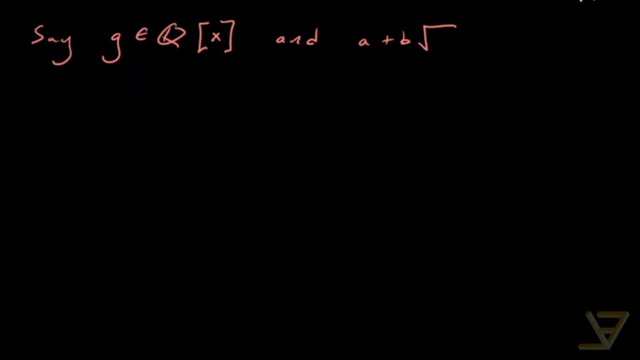 And a plus b square root of d, with a in the rationals, b in the rationals and d in the rationals that are positive, Then what we find is that if this number is a, 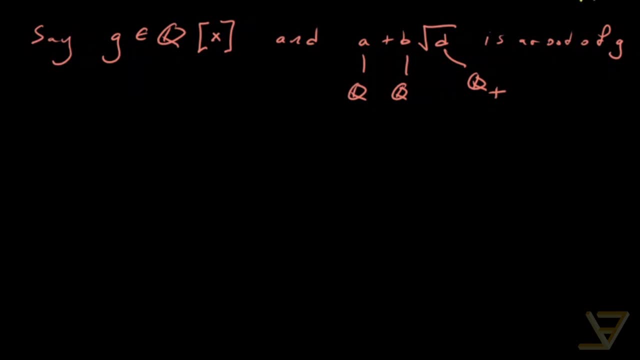 root of g, then it's radical conjugate: a minus b. square root of d is also a root of g, And this is true because of the same properties that we used earlier, But we have to prove it separately. 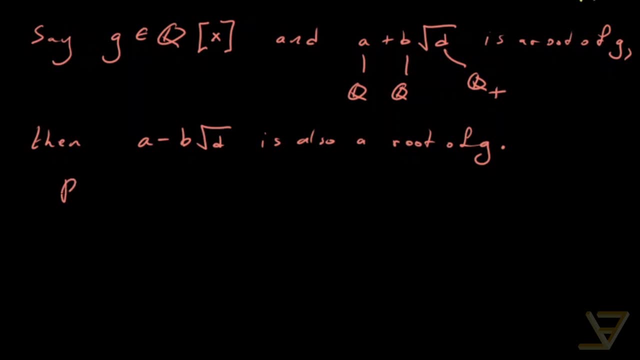 What we find is that if radical conjugates are denoted by, let's say, a plus a plus b, square root of d, and we put an underline underneath it, then that's equal to a minus b. 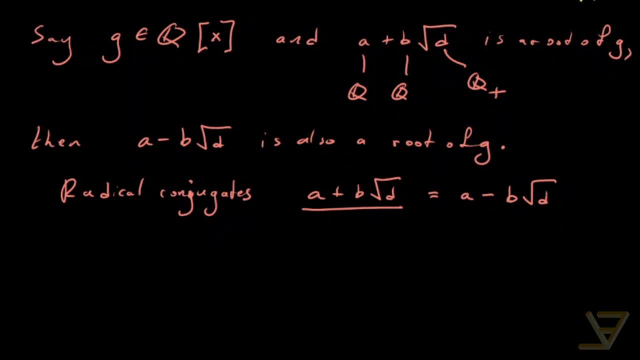 square root of d. So what we're going to find is that a plus b square root of d, plus, let's say, x plus y, square root of d, If we do an underline for the whole thing. 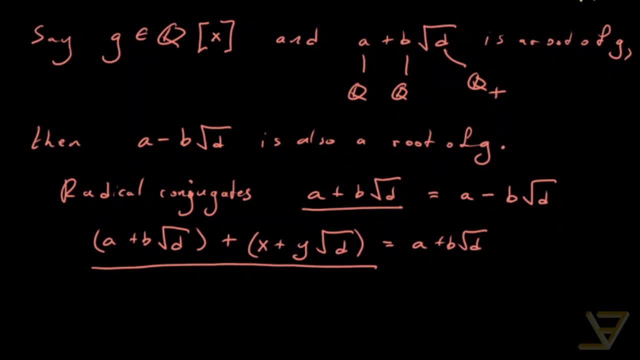 it's equal to a plus b, square root of d, underline. plus x plus y, square root of d, underline. And same for multiplication. And finally, the property that we need. it's analogous to the fact that the conjugate